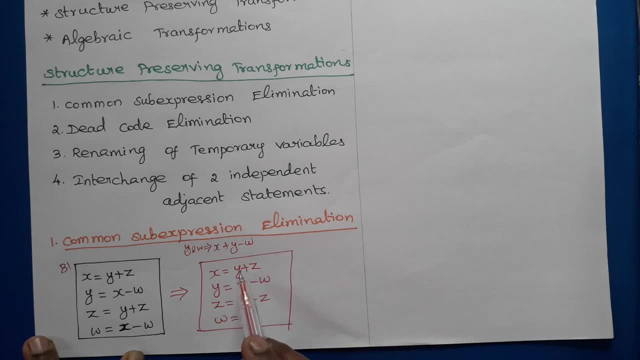 to definitely be using common sub-expression. So the expression appears same, That is y plus z. but this second statement redefines y. The y is recomputed in the second statement, right? Therefore this y is not equivalent to this y, So z is computing x minus w plus z. So these are not common sub-expressions, So it. cannot be eliminated from the base block. Now I am going toAssume that the husband should know the opposite of x. So, for example, either i is greater or greaterwe can replace y. Don't worry that we don't have much freedom of possibility. We can replace, but we can. 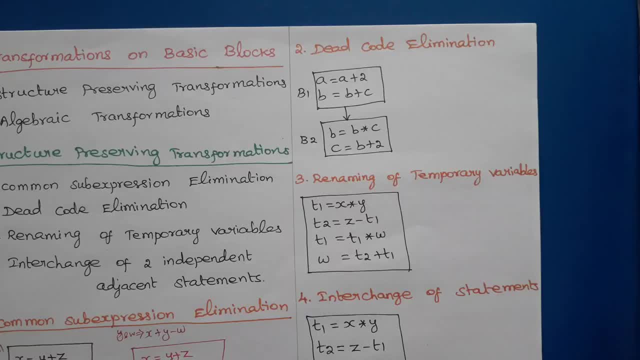 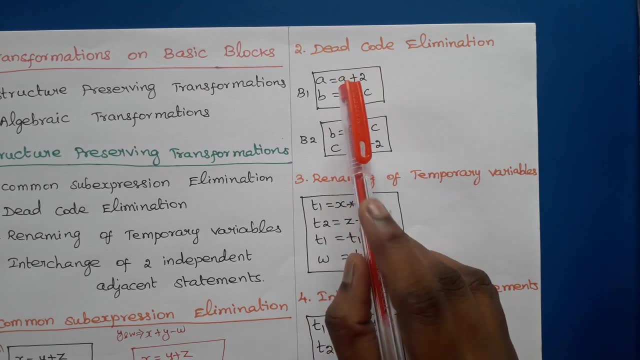 also now vienenc wallet index, and then we get this a little NPK, we can also. there is you block. second transformation is dead code elimination. dead code: a variable is said to be dead if it is not subsequently used in other basic blocks or it is not. 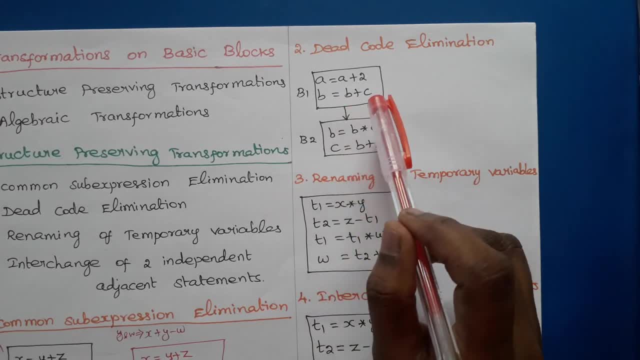 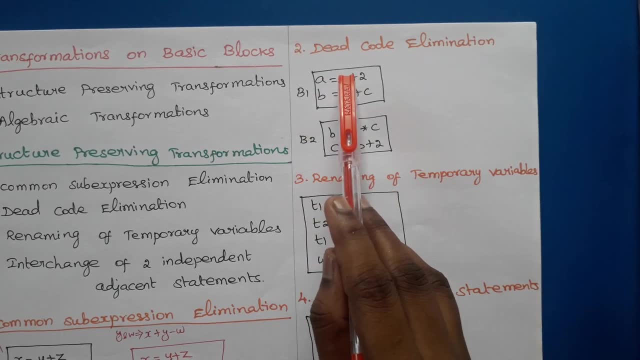 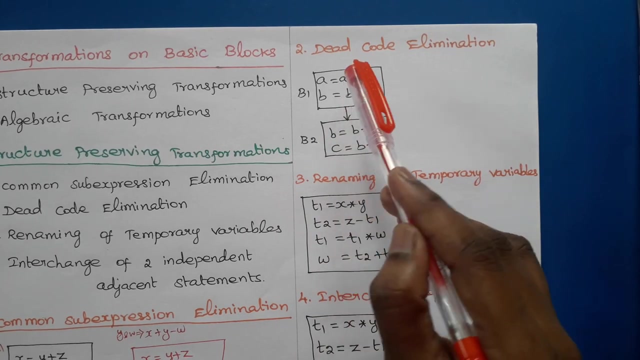 subsequently used further. so here in this example assume that b2 is a final block, final basic block. so here a is computed as a plus 2 and b is b plus c, and here also b equal to b star c, c equal to b plus 2. so this a is not used. 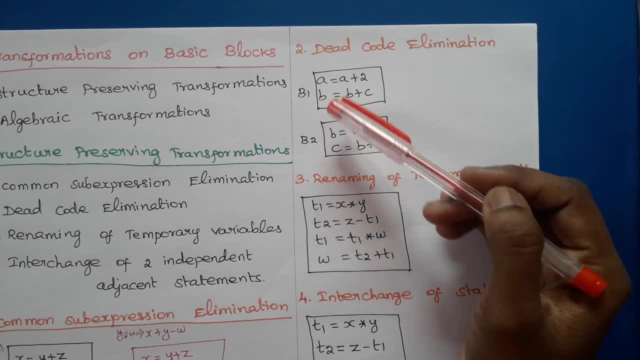 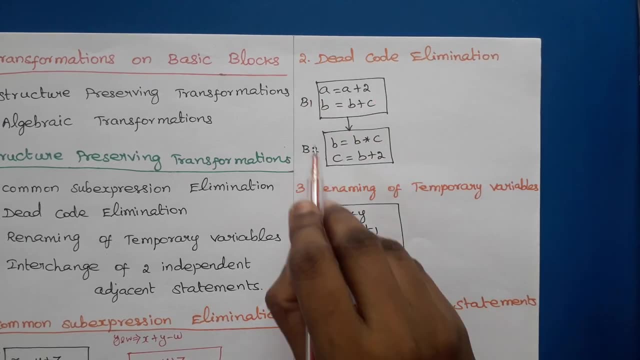 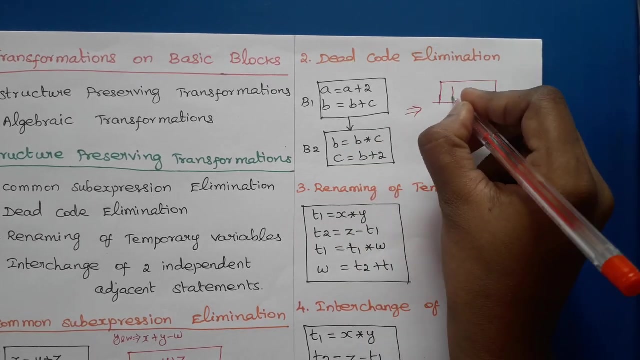 in the basic block to final block 2. so after this point a is not used. so we can say that this is the dead code, so it can be safely removed without changing the value of the basic block. so after eliminating dead code we will get B equals B plus C alone in basic block 1 and there is no 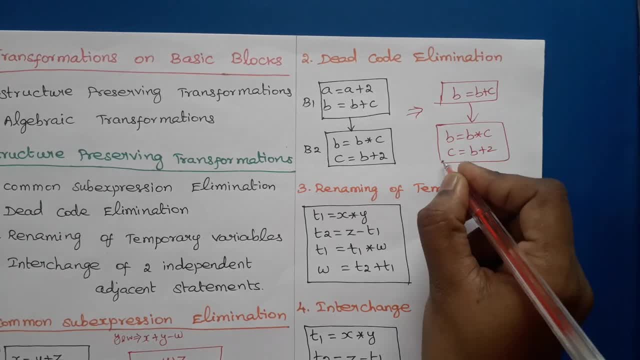 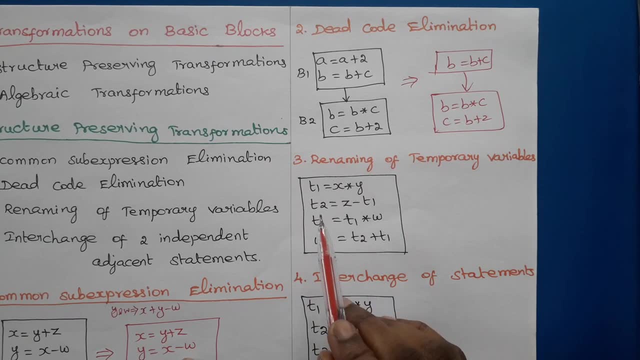 change in basic block 2. so this is called as dead code elimination, then renaming of temporary variables. renaming means a temporary variable can be renamed with another temporary variable. so for example, consider this basic block here: t1 is equal to x, star y, t2 is z minus t1. 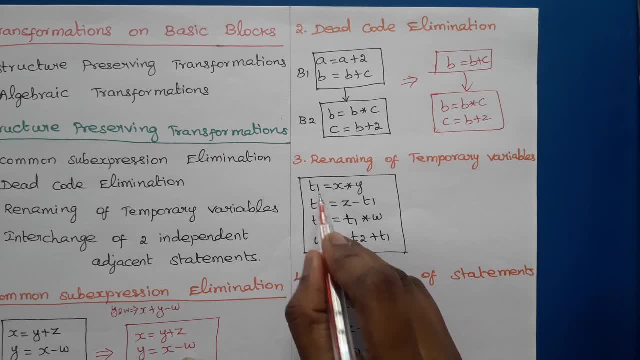 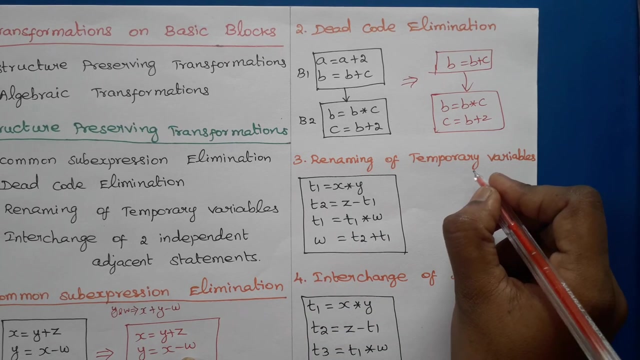 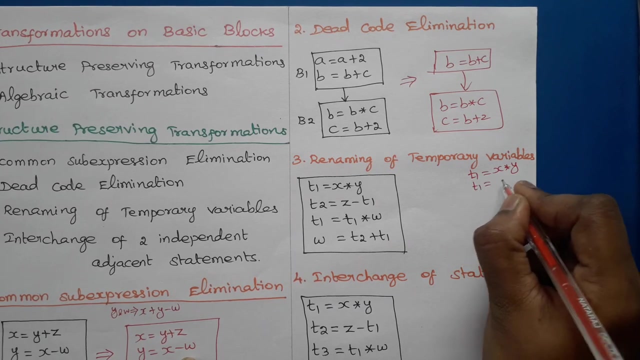 and t1. here again, t1 is evaluated as t1 star w, and that is w is multiplied with x star y star z. so t1's value is changed here. okay, so previously t1 was x star y. after executing the third statement, t1 is changed to x star y star w. okay, so. 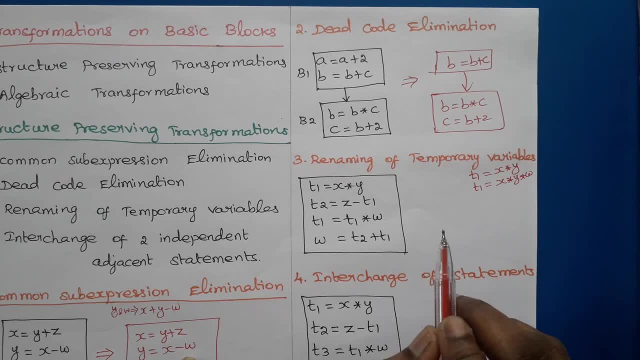 now the current value of t1 is x, star y, star w, but sometimes we want to. we want to retain x, star y also. this temporary variable also needed by some other block. so if we want to retain t1 also means instead of this t1 we can introduce a new temporary variable, so we can rename this. 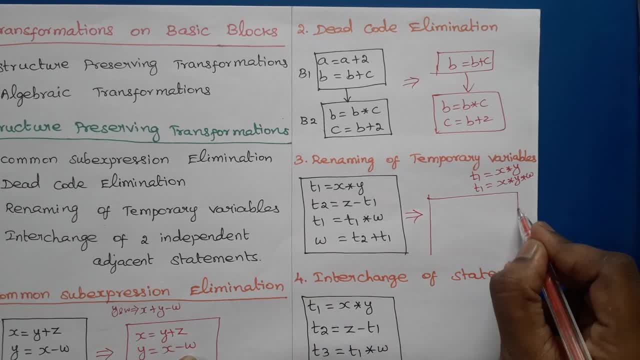 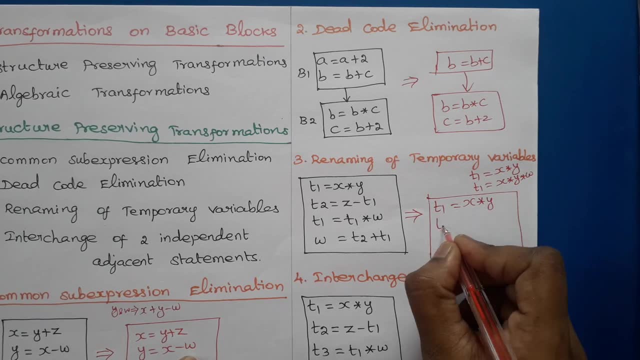 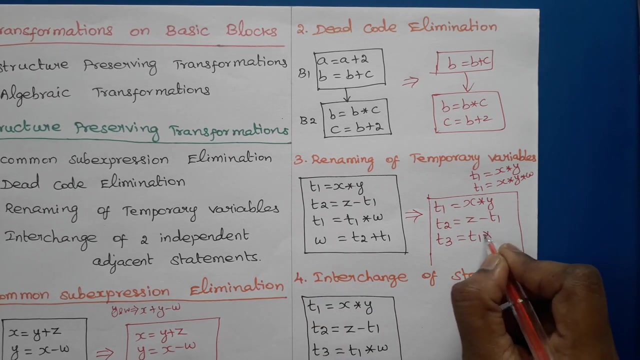 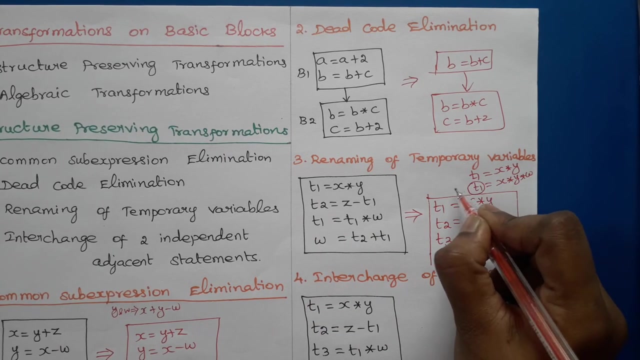 temporary variable. so if we want to replace t1 into t3, t1 is x star y, t2. t3 should be substituted here. t3 equals t1 into w. so this t3, this statement, is evaluated in t3. so instead of t1 we are using t3. so if we want to use x star y star w in further statements, 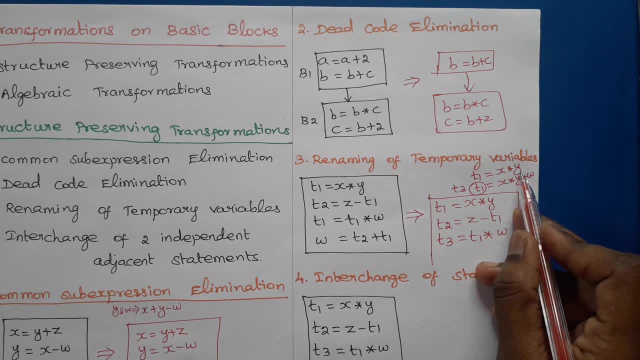 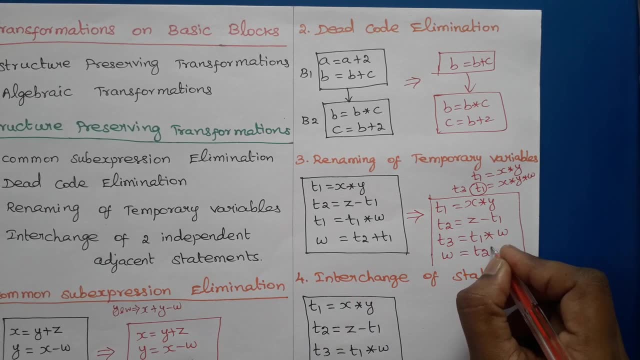 basic block we can use t3. x star y should be computed means we can use t1. then w is equal to t2, plus here t1 represents this t1, so that is renamed as t3. so we have to write t3 here. so if 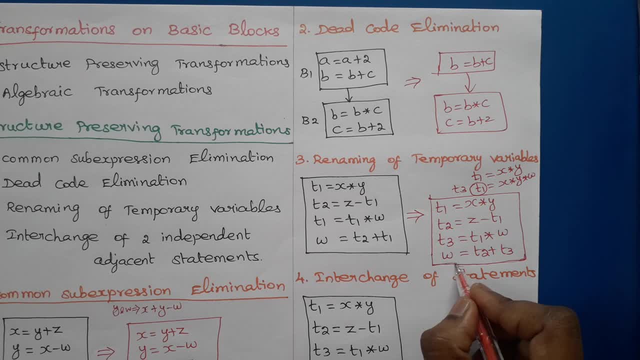 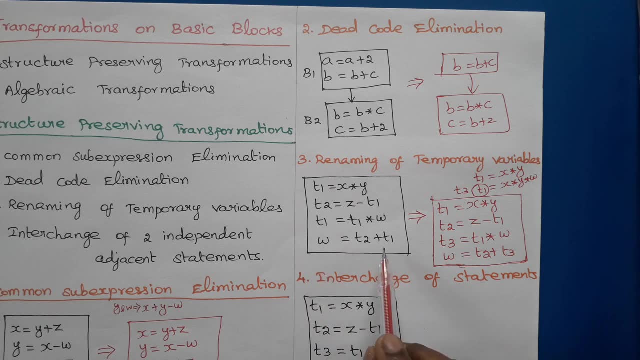 we want to rename a temporary variable into another temporary variable, we have to replace all the uses of that temporary variable with a new name here, after. after this point, after the fourth statement, all the t1 should be renamed as t3, then only the meaning or the value of the. 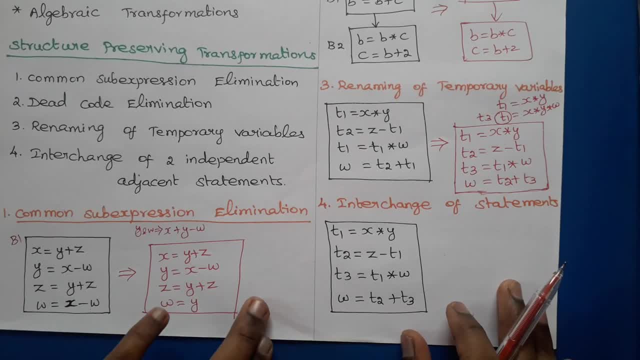 basic block will not be changed. so this is a renaming of temporary variables. then the final structure perceiving transformation is interchange of two independent adjacent statements. in independent statements means the, the, the. the two statements are not depending upon anything one each other. so for example here: t1 is x, star y. 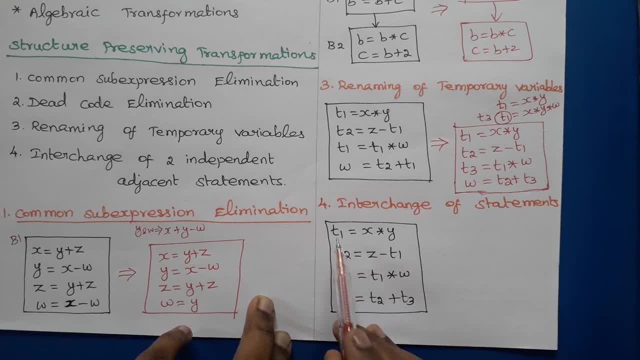 t2 is computed as z minus t1, so it depends on the previous statement, t1. so these two statements are not independent statements. now consider t2 and t3. t2 is z minus t1. t3 depends on t1. also t1: star w. 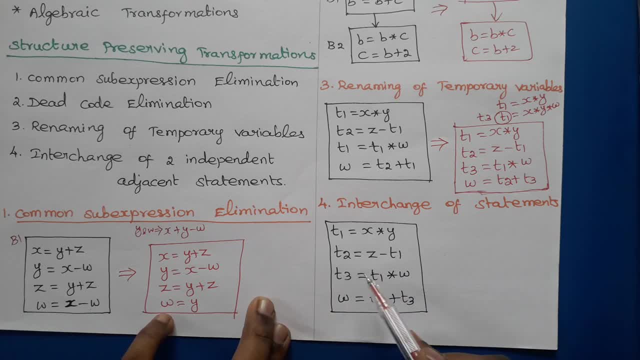 so these two are the independent statements. so we can say the statements are independent if neither z nor t1 is t3 here. if t3 is used in the right hand side of the this expression, then it is not dependent, it is not independent statement. similarly, here t2 is used means this is not independent statement. so now these two are the. 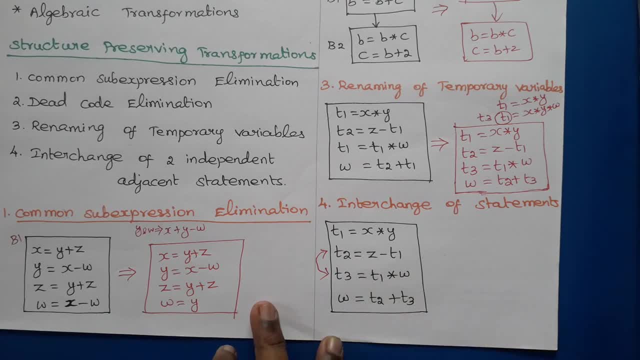 independent statements, so we can interchange these two statements without, uh uh, changing the value. similarly, uh, if you consider the final statement, here t3 is used, so this is not a independent statement. so only independent statements in this block are t2 and t3, so we can interchange these two. 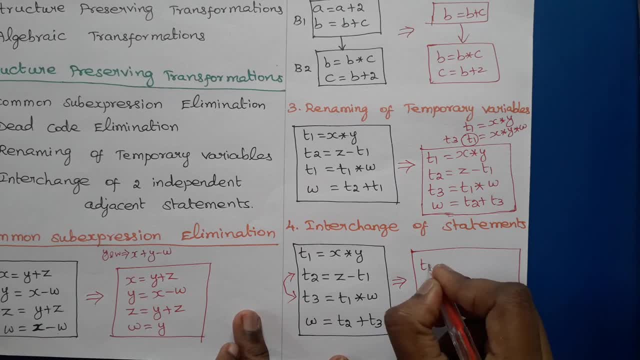 so t1 is equal to x star y, t3 is equal to t1 star w, t2, z minus t1 and w is t2 plus t3. so now the meaning of the basic block is not changed. so, based on our usage, we can use the interchange of statements. 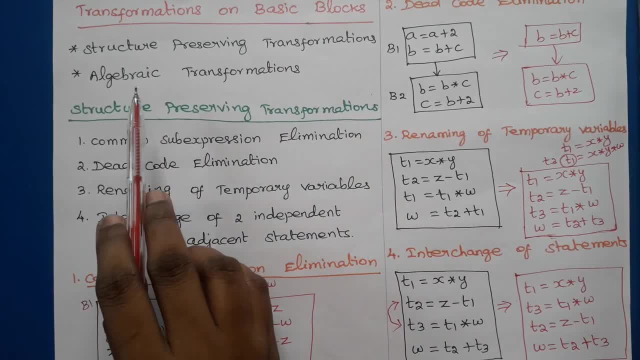 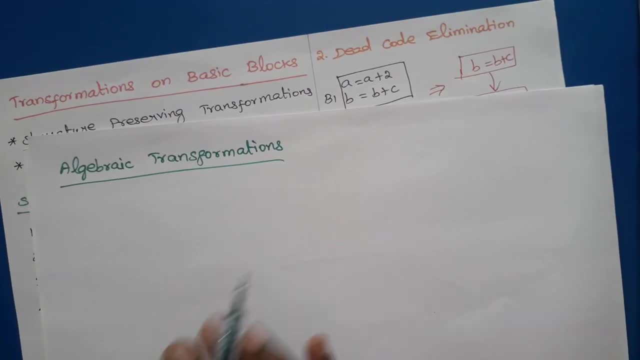 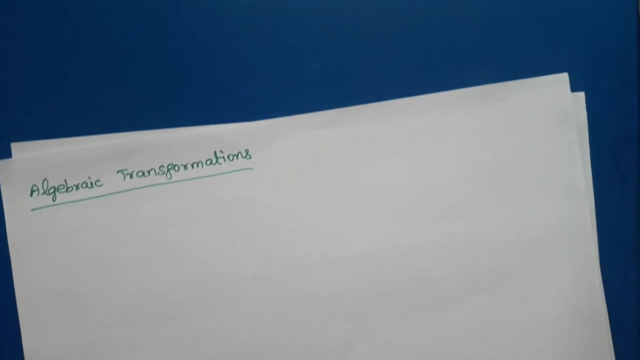 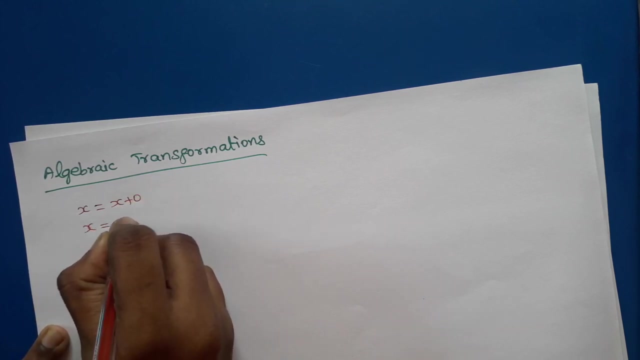 then second type of transformations on basic blockers: structure preserving transformation. sorry, the second type is, uh uh, algebraic transformations. so several algebraic transformations can be performed on the basic block. some examples are suppose if the basic block is having x equal to x plus 0 and x equal to x plus, 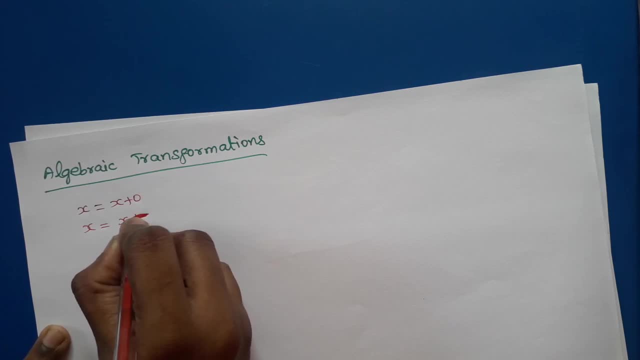 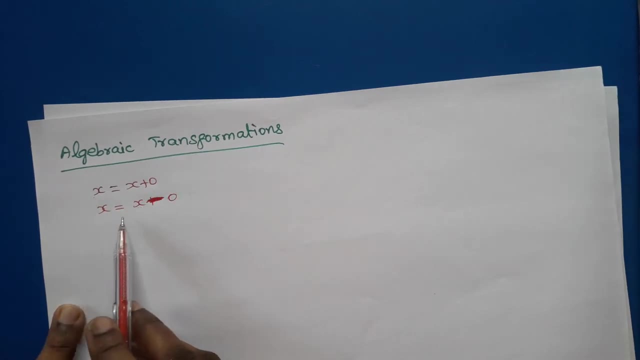 um x minus 1, x minus 0. so consider these two statements: x equal to x plus zero, or the basic block is having x equal to x minus 0 means the value of x is not changed here. so these two statements can be completely removed from the basic block without changing the value of the. 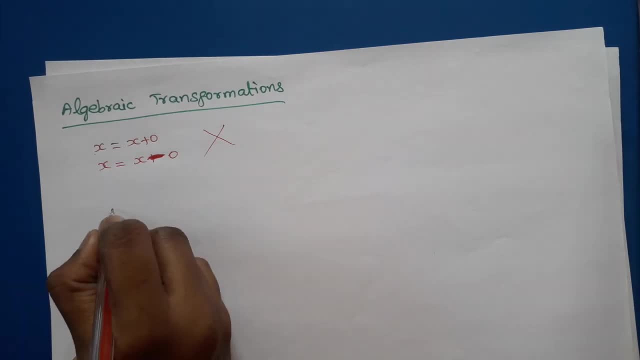 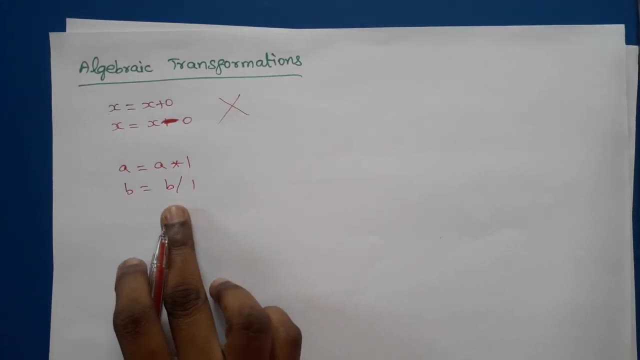 basic block. these two statements can be completely removed. similarly, a equals a star 1 and b equals b divided by 1. here also the meaning is not changed. the value of a is not changed here, b is not changed here. so these type of statements also can be removed from the.